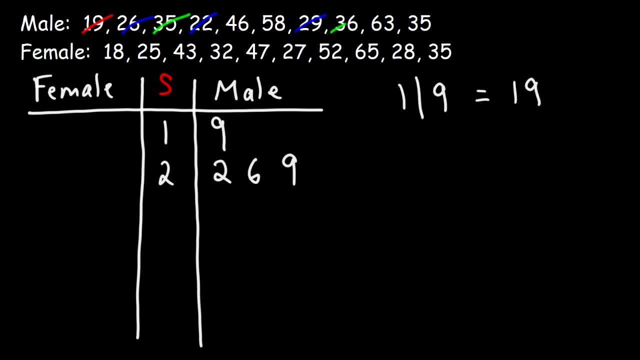 40,. we have these two numbers 35 and 36. And there's another 35. So let's write 3, and then 5,, 5,, 6.. Now in the 40s I only see one number: 46. So we just got to write 4, and then 6.. Next we have 58. So 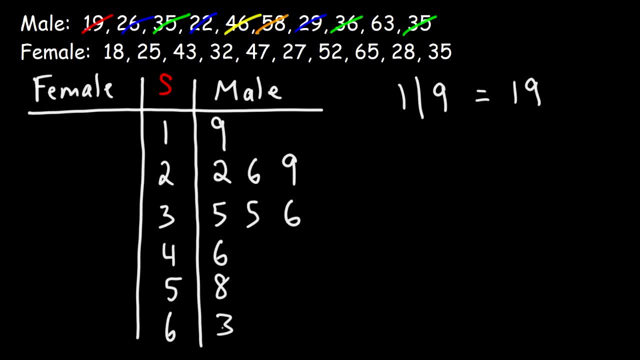 we could just write 5,, 8. And the last one is 63. So those are the ages for the males. Now let's move on to the ages of the females. So we're going to use the left side. So the first one that we have here is 18.. So all we need to do is put an 8. 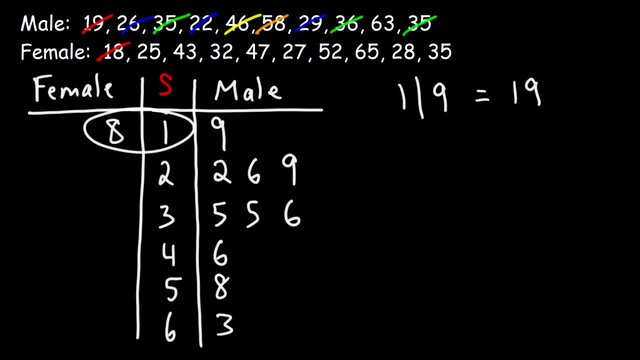 on the left side, So this corresponds to 18.. You have to read it this way. It is kind of weird because typically I don't know about you, but I'm used to reading things from left to right, So with the side-by-side. 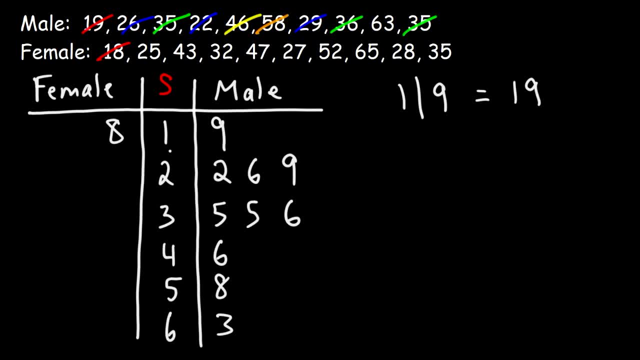 stem-and-leaf plot. you also have to read things from right to left, So just keep that in mind. Now let's move on to the next set of numbers. We have 25,, 27,, 28.. So the first number in a set in order will be 5, and it's like writing it. 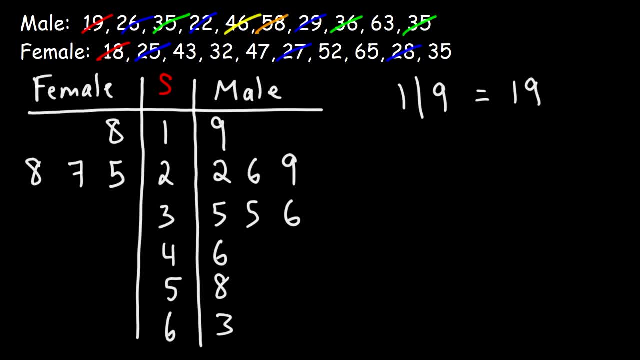 backwards, and then 7, and then 8.. So you need to increase the numbers in this direction Now. next we have 32 and 35. So we're going to write 2 and 5 in the third row. After that we have two numbers in the 40s: 43 and 47. And then we have 52, and 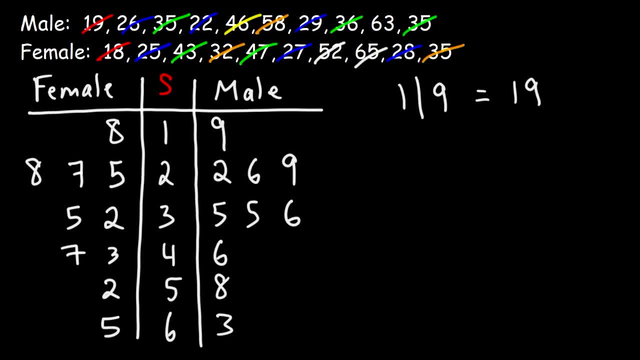 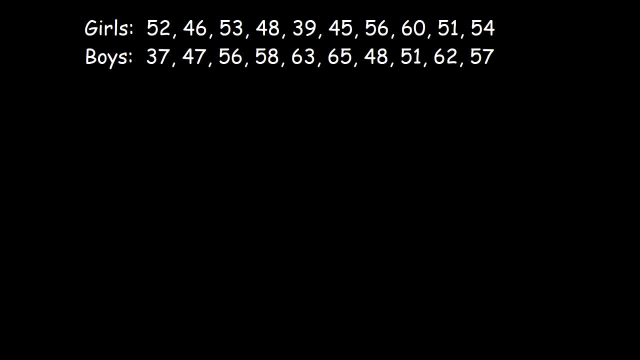 finally, 65. So that's how you can make a side-by-side stem-and-leaf plot. For the sake of practice, let's try another example. Feel free to pause the video if you want to work out this example. So what we have here are the heights of girls and boys.